25,, 26,, 27,, 28,, 29,, 30,, 31,, 32,, 32,, 33,, 32,, 33,, 34,, 34,, 35,, 36,, 37,, 38, icy. 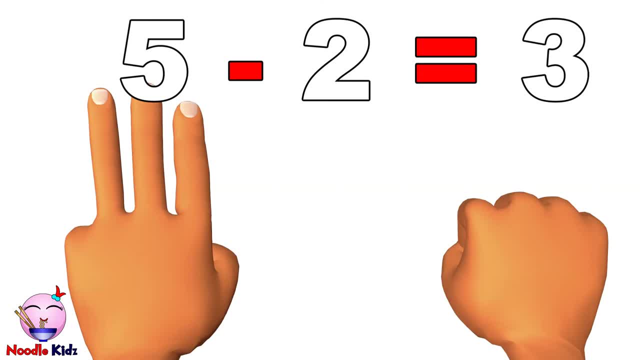 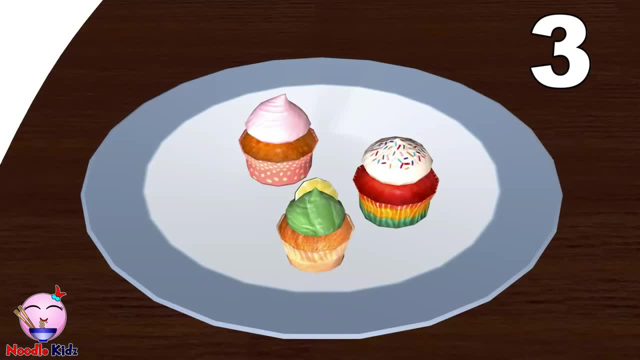 Three, Yes, 5. take away 2, equals 3.. Now we at only one four. we have two, three, two, three, 3, yes, Five. take away two, equals 3.. There are three cupcakes on the table. 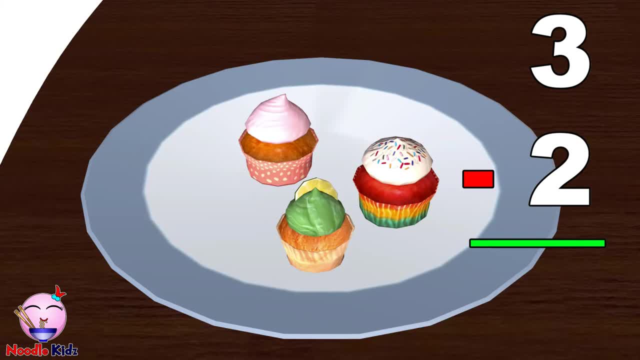 If you take away two, how many will you have left on the table? You will have one cupcake left on the table: 3 minus 2 equals 1.. You can all believeakovish Brazil. Take two, Yes, 5. take away 2 equals 3.. 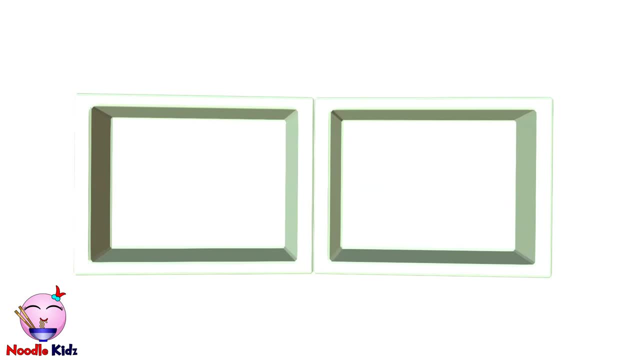 There are three cupcakes on the table. There are three cupcakes on the table. You can also use boxes or shells system for subtraction. What is 6 minus 4?? First write down 6.. Then draw two boxes or shells next to each other under the number 6.. 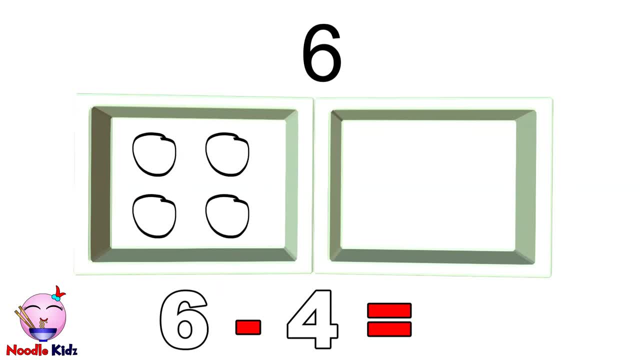 Draw four circles in one box. How many circles should we have in the next box? Let's count the while pointing the circles in this box and drawing more circles in the next box: 1,, 2,, 3,, 4,, 5,, 6.. 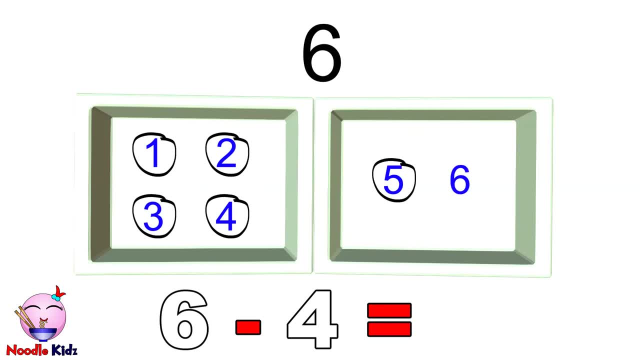 You need to draw circles on number 5 and 6.. This means you need two more circles. There you have it. You need two circles to complete the equation. This means 6 minus 4 equals 2.. Let's try again. 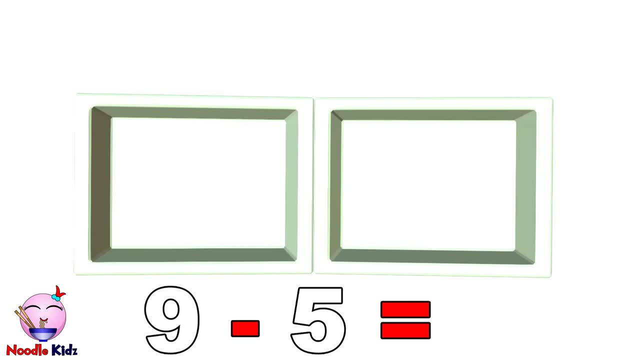 What is 9 minus 5?? Write down number 9.. Draw two boxes below number 9.. Draw five circles in the left box. Start counting while writing down the numbers 1,, 2,, 3,, 4,, 5,, 6,, 7,, 8,, 9..